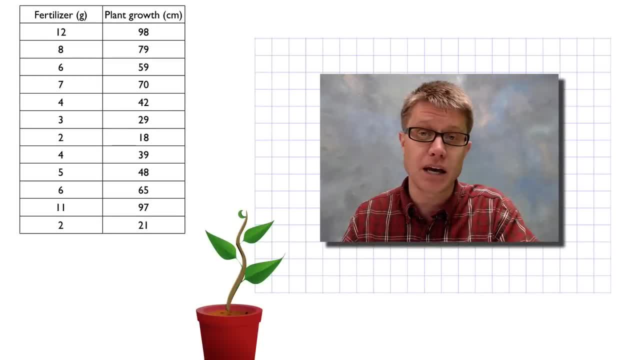 the best place to start. And so let's say I give you the following data. Let's say I do a lab where I vary the amount of fertilizer that I'm giving plants and then I measure how high those plants grow. And so the independent variable in this case is going to be the fertilizer. 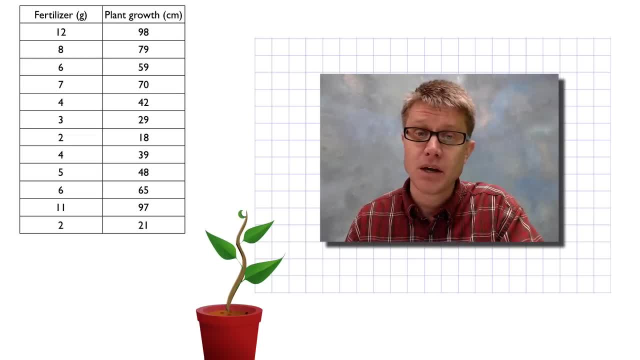 and the dependent variable is going to be the growth of the plants, And so you could pause the video if you want to. right now, You could try to make a graph of this data, and then you could come back and look at the important parts of the graph and how I set. 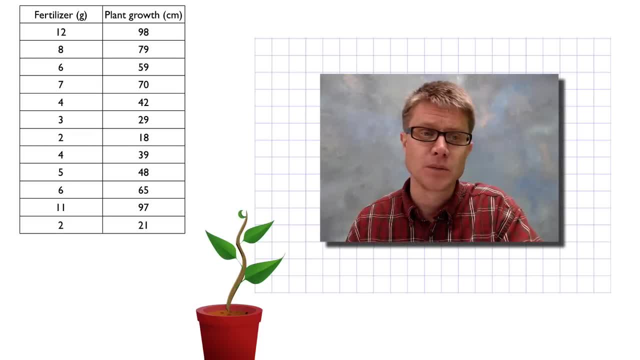 it up, Or you could just watch me and then, when you're done, try a graph of your own, And so the first thing you want to do is figure out what kind of a graph you're going to use. In this case, I'm going to use a scatter plot, Because I'm looking at the correlation between 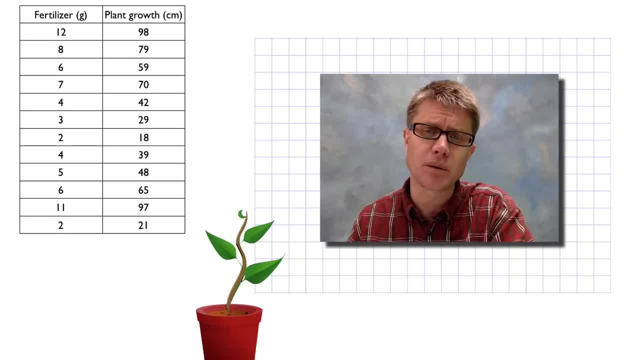 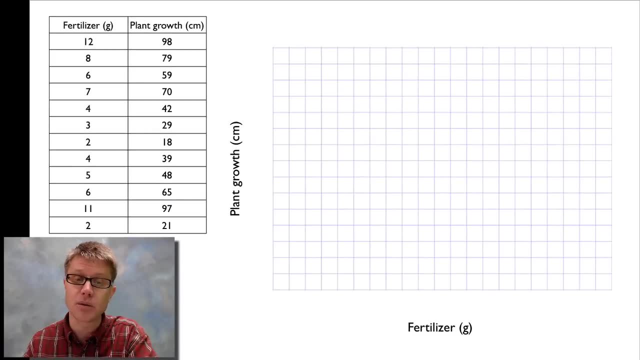 two number sets. The next thing I want to do is I want to make sure I set up my axes in the right way, Since I'm varying the amount of fertilizer. I want that to be on the x-axis and I want plant growth to be on the y-axis. The thing you change will be here And the 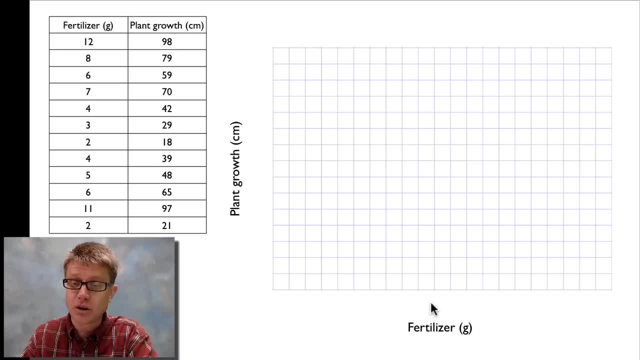 thing that you measure will be here. Notice that I've also put what I'm measuring and then the units that I measure it in. So fertilizer is going to be measured in grams, and I put that in parentheses. Just likewise, plant growth is going to be on the y-axis, and then I put: 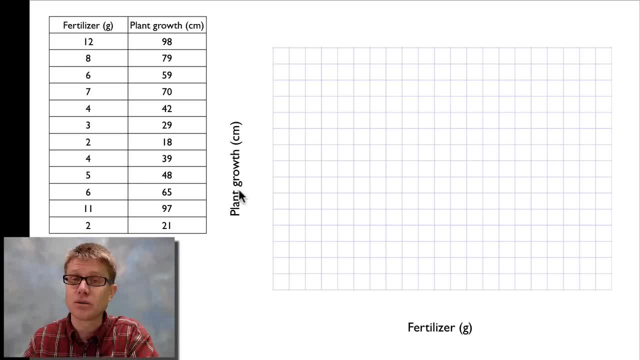 that Measuring in centimeters. Next thing I want to include is a good title, And so I could look at the relation of fertilizer to plant growth. If I knew more about this lab, like the type of plant or the time period when it was done, I would include that in my title. 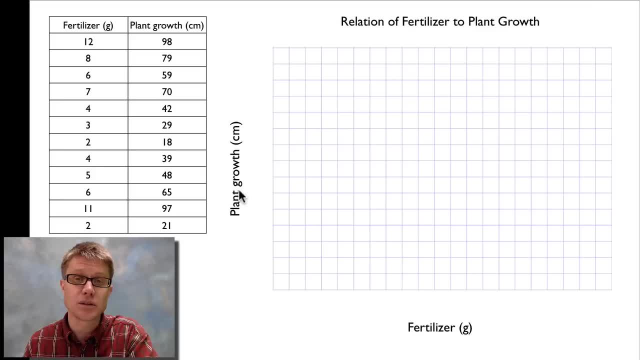 as well. Make sure that you can look at the title and you should be able to label the axes just based on that. You shouldn't have the title that's, for example, just plant growth. You want to have as much information in that title as you can. Next thing I want to do: 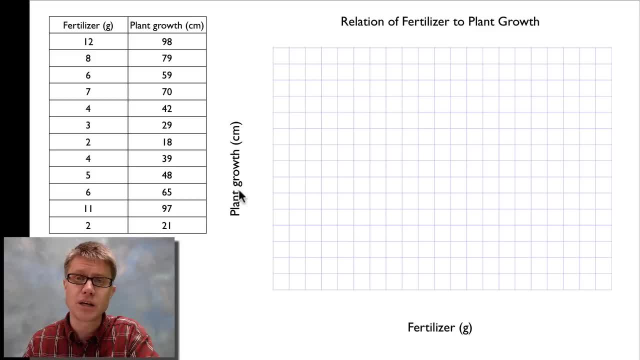 is, I want to put numbers and I want to put tick marks or major grid lines on both the x and the y-axis. This is hard to do, And so let's say you're doing a test and you're given this amount of graph paper. You want to make sure that you use all of the graph paper And that's going to. 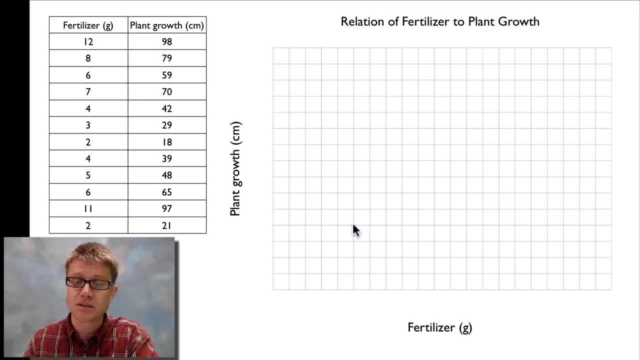 give us a better graph And it's going to allow us to look at patterns in the data, And so this is sometimes difficult. First thing I want to do is count the number of squares, And so I count the total number of squares, And it's 21 squares. And then I look 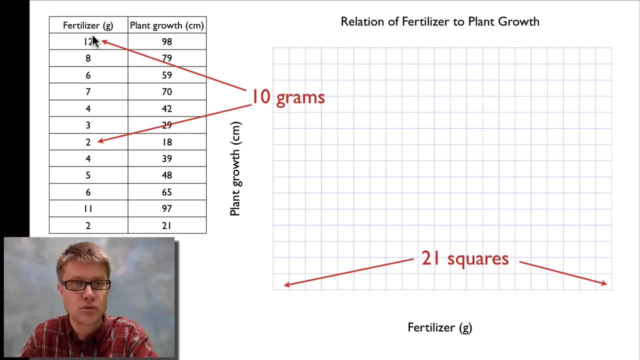 at the range, And so you can see here that my fertilizer values go from 2 to 12. And so I have a spread of 10 grams that I want to make sure I'm able to graph. Now, students have a tendency to want to put the number 0 here, But since 0, 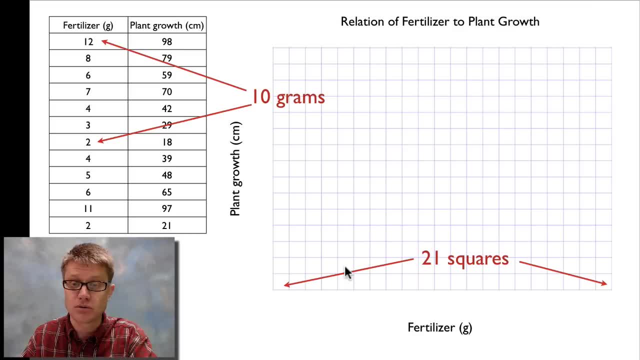 is not in my data set. I don't want to include 0 on my graph, I want to use all of the graph paper, And so a quick way to do this: if I divide the number of grams by the total number of squares, that tells me basically how many grams per square, And so I could start here. 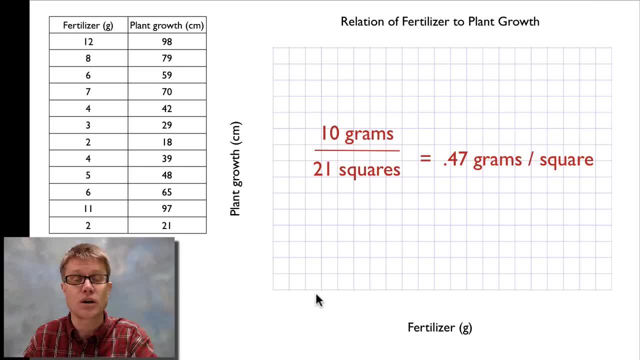 this being 2,, this being 2.47, and then just move across like that. But you can see it's going to be really unwieldy. It's going to be a bunch of decimal values. It would end exactly at 12, but it's not going to look that nice. And so, since I'm less than 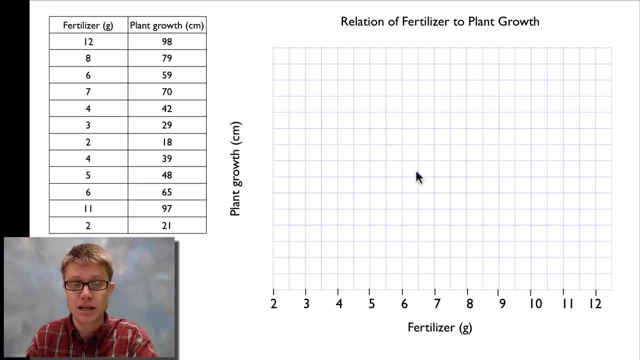 0.5,. I could simply round up to 0.5. And so I could label it across the bottom as 2, 2.5, 3, 3.5 and 4.. And so I've labeled all of the whole numbers across the bottom. I didn't. 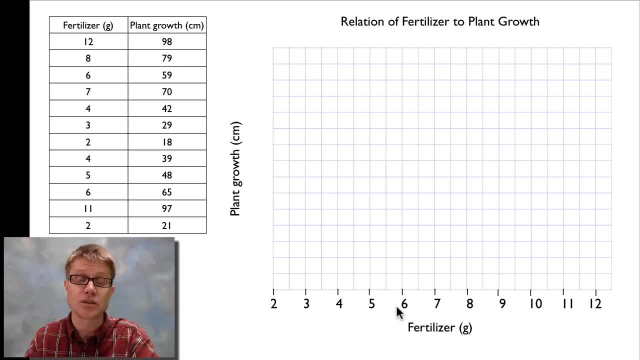 have to put all of those there, but I at least have to have two or three numbers so that you can figure out what the scale is going to be. Now, let's go, try and do this. I'm going to go ahead and do this. I'm going to go ahead. 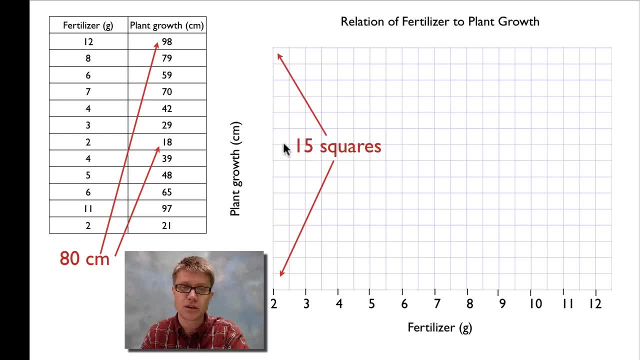 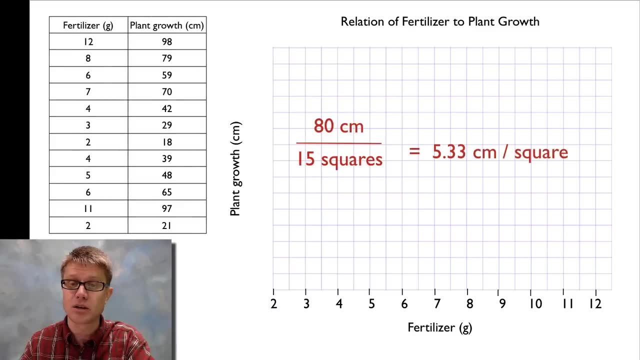 and do the y-axis, or plant growth. I count 15 squares here on my graph paper And I've got a range of 80 centimeters of plant growth. So likewise I could divide that 80 centimeters by the number of squares and that's going to give me 5.33 centimeters per square. So 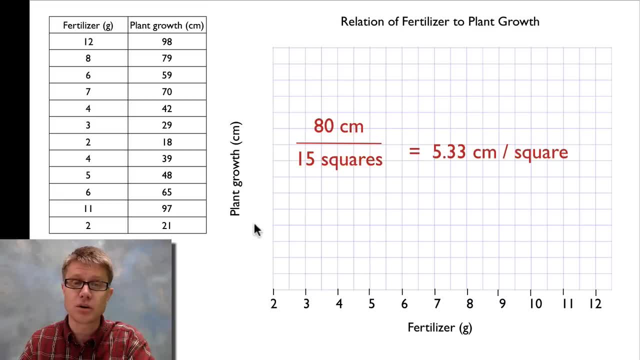 if I were to round down to 5, I wouldn't have enough room to put all of my data here on the side, And so what I can do is I can round up And I can say that maybe every one of these grid lines is going to be 6 centimeters. 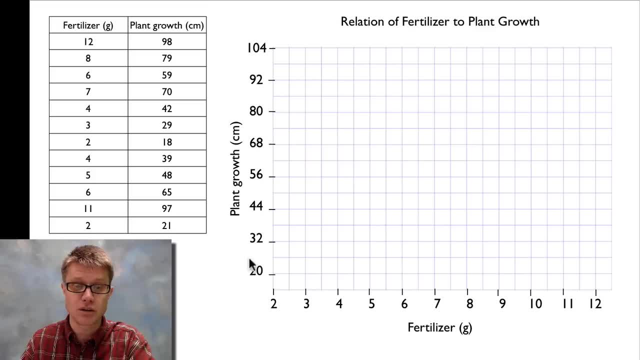 And now I put my label, my axes, on here. I want to make sure that I can go all the way from 18 up to 98.. So each of these is then going to be 6 centimeters, And so I can show all of my data, So every. 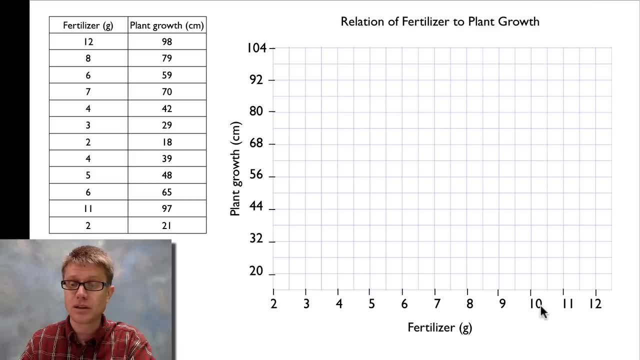 two is going to be 12.. And so you want to make sure that it's a linear labeling of the x and the y-axis. The next thing I want to do is I want to graph my data. Well, what's my first data point? Fertilizer of 12.. So I'm going to go all the way over here to 12.. 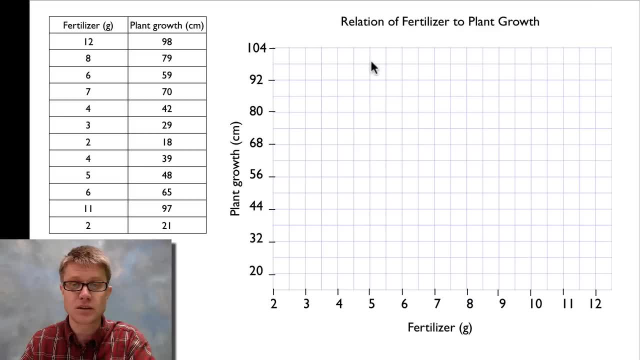 And then I'm going to have plant growth of 98. Well, if this is 92, that means that this is 98. So my first data point should be right there, And so now I'm going to put all the other data points from my graph, So I'm going to fill those in with dots. Now you can see. 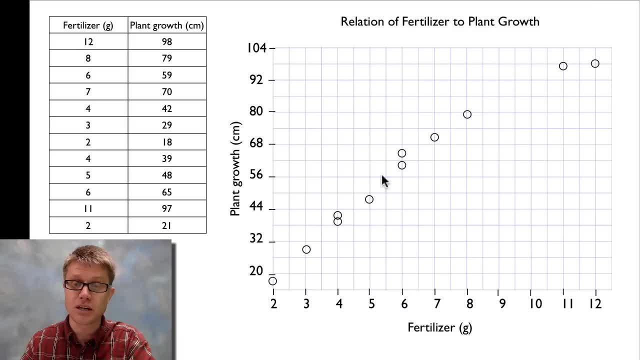 that there were some times when I had the same amount of fertilizer but two different types of plant growth, And that's fine. One thing I don't want to do right now, if I'm doing a scatter plot, is I never want to connect these lines Because those are different plants. 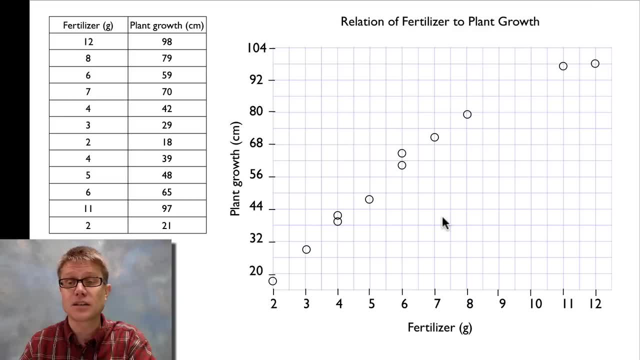 And so that wouldn't make any sense. I'm almost done, though. What's the last thing that I'm missing right here on my graph is going to be a graph, So I'm going to go all the way over here and I'm going to put a line of fit, And so a line of fit is going to be a. 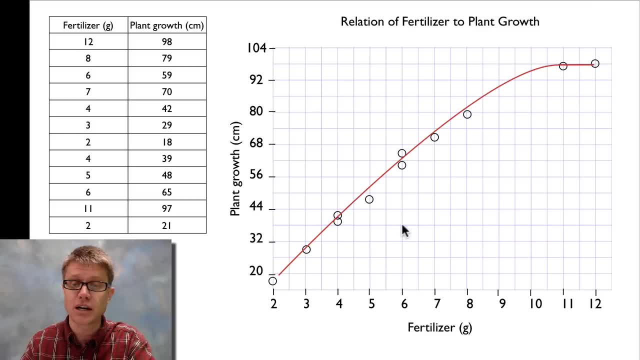 line that represents the average of my data. It doesn't always have to be a straight line. You can see in this case that as I increase the amount of fertilizer, it starts to stabilize up here at the end, And so that's going to be my line of fit. We don't want to extend.